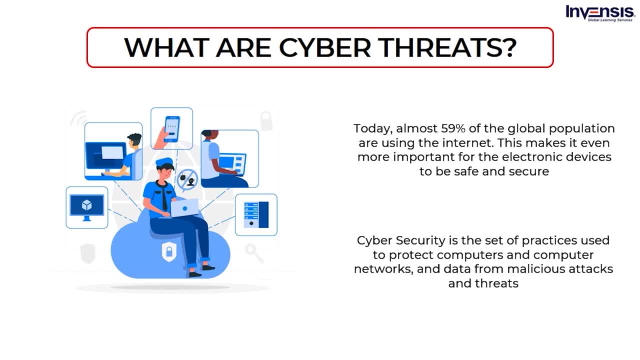 be safe and secure. Hackers have started coming up with ways to gain unauthorized access to the internet. This is a great way to prevent cyber security threats. Cyber security is the set of practices used to protect computers, computer servers, mobile devices, various electronic systems, communications and computer networks and data from malicious 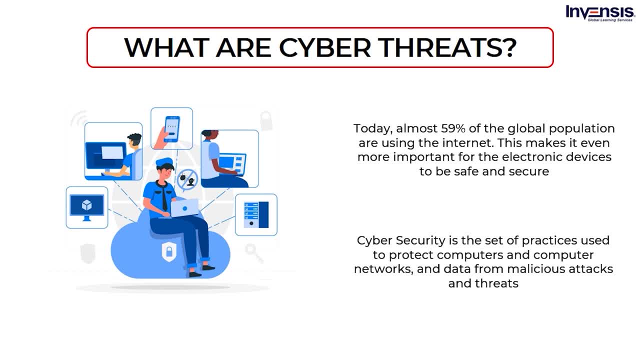 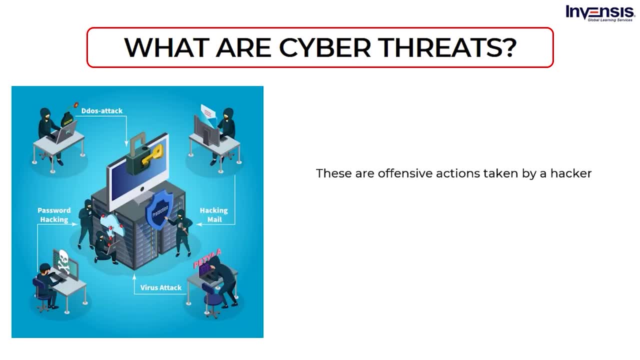 attacks and threats. It is also known as information technology security or electronic information security. A cyber threat is an offensive action taken by a hacker or unauthorized individual or a group of individuals. These malicious attacks and threats are called cyber attacks or cyber security threats. A cyber threat is an offensive action taken by a hacker or 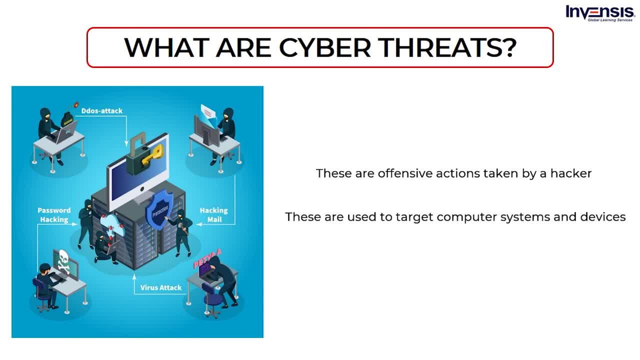 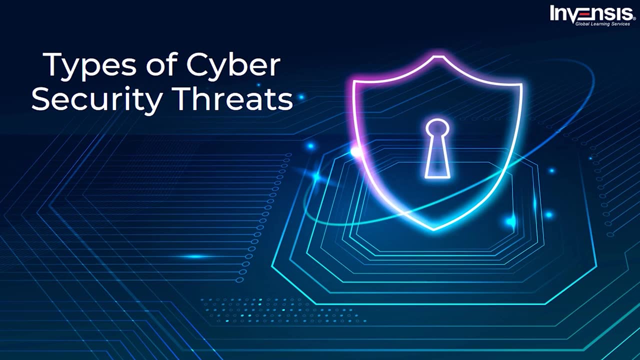 unauthorized individual or a group of individuals. These malicious attacks and threats are called cyber threats. They target computer systems, IT infrastructure, computer networks, mobile devices and other computer devices. They use different methods to break into, steal, damage or alter crucial data and information. Let us now look in detail at the types of cyber security. 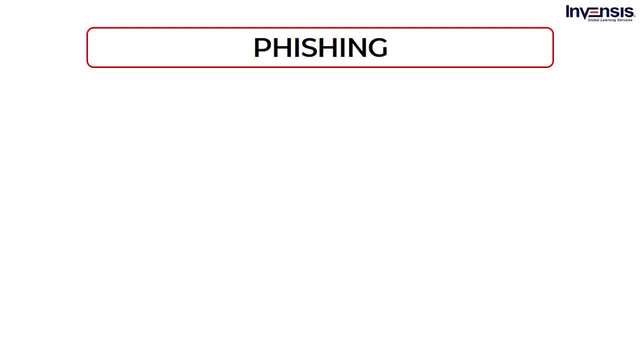 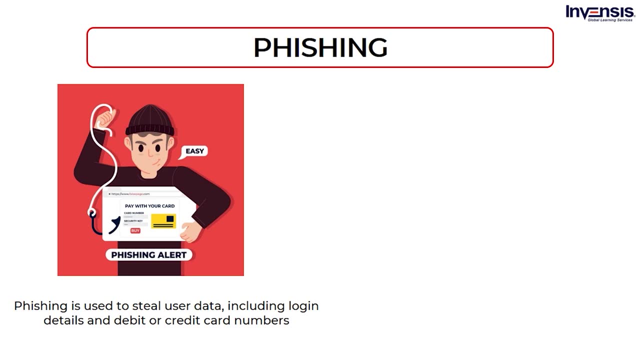 threats. The first type of cyber attack is called phishing. Phishing is one of the most used types of cyber attacks. The attackers by this method try to get access to personal information like login credentials, data and information. The attackers by this method try to get access to. 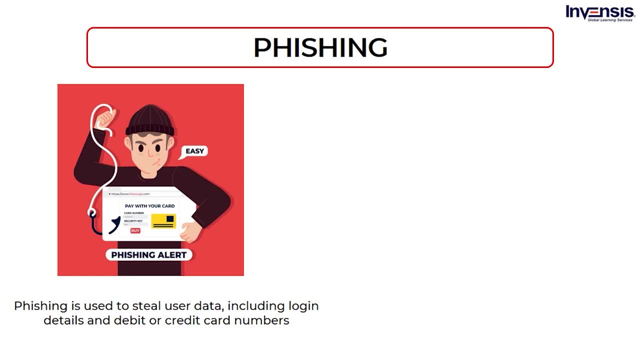 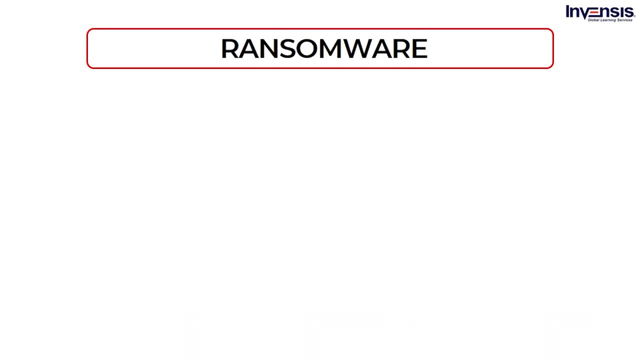 credit card details by pretending themselves as concerned competent authorities. Phishing is executed mainly through emails, messaging and phone calls. The next type of cyber attack is called the ransomware. In a ransomware attack, the user is compelled to remove all of their data and 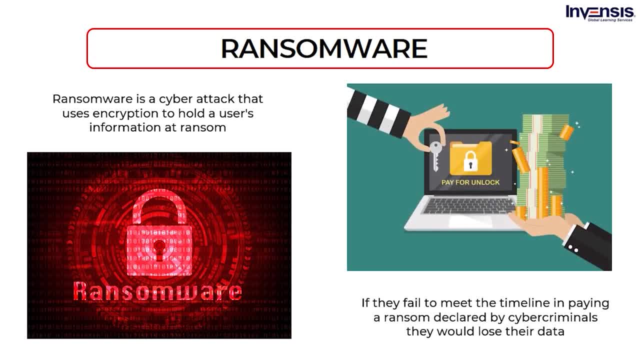 information from their system if they fail to meet the timeline in paying a ransom declared by cybercriminals. In spite of all this, there is no guarantee as to whether paying the ransom would secure their data or not. Let us now look into a ransomware attack. The ransomware attack is a 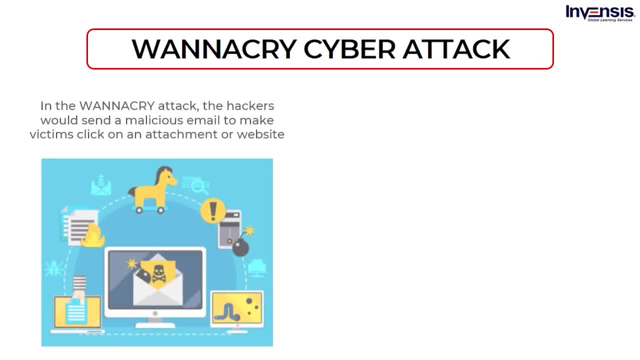 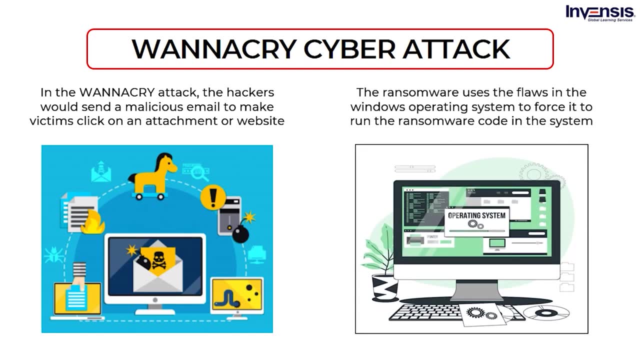 recent 2017 ransomware attack called WannaCry. In the WannaCry attack, the hackers would send a malicious email to make victims click on an attachment or visit a website. The ransomware uses the flaws in the Windows operating system to force it to run the ransomware code in the system. 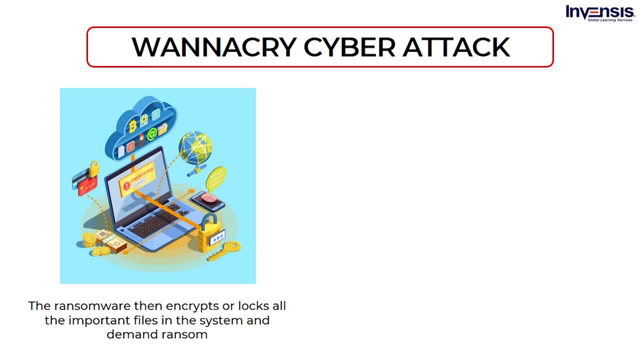 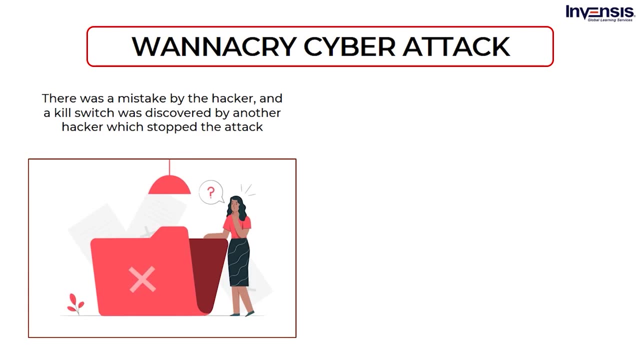 The ransomware then encrypts or locks all the important files in the system and demands a ransom in the Bitcoin cryptocurrency. The WannaCry ransomware uses the operating system flaw to replicate itself and spread around the computer network. The hackers, however, made a mistake. A kill switch was discovered by another hacker. 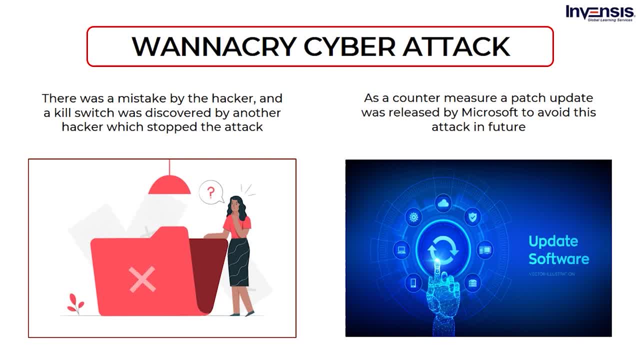 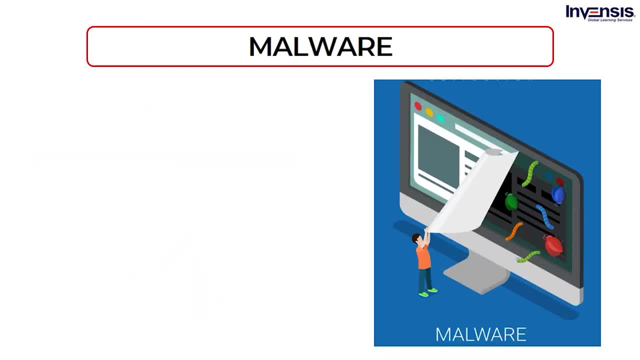 which helped in overcoming this attack. Microsoft also released a patch update. Both these measures help the users to regain access to their documents. The next type of cyber attack is called malware. Malware's short form for malicious software is a code or file created by hackers to be delivered over a computer network. It is used to infect. 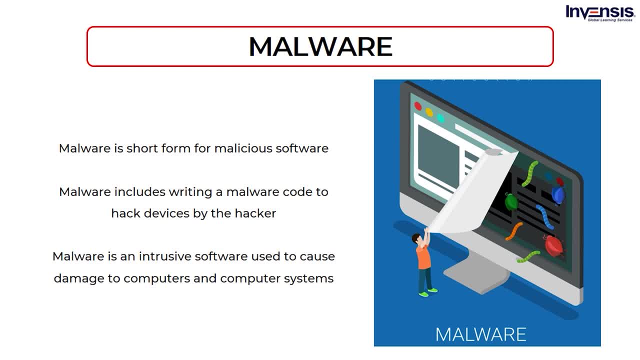 steal or to gain control over a system or network. to gain an authorized access In a malware cyber attack, the hackers create a malware code to hack any electronic or digital device. These devices can be mobiles, computers and laptops. to obtain unauthorized 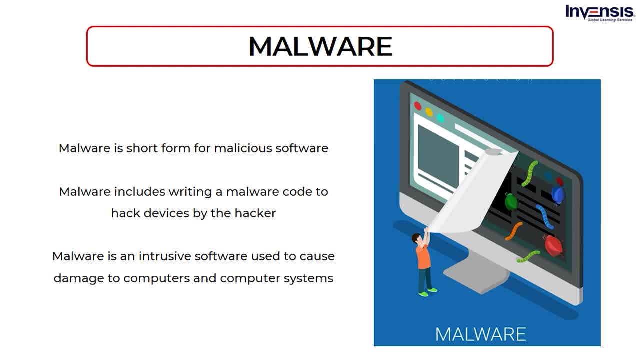 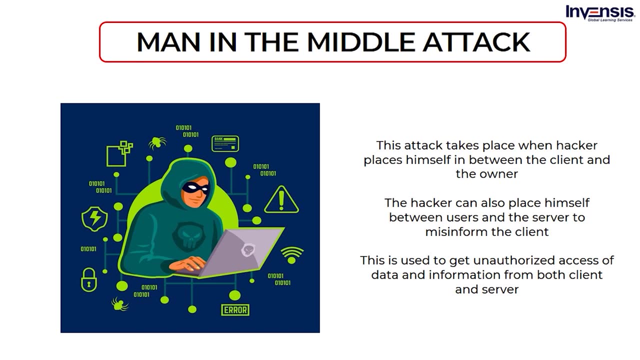 access to sensitive information. It takes critical expertise to create the malware code and is extremely dangerous for the users who are prone to such attacks. Malware is an intrusive software used to cause damage to computers and computer systems. Now we are now going to discuss the man-in-the-middle attack. A man-in-the-middle attack. The malware is a software used to attack users who are prone to sic smiling. If you use malware, hackers will always be able to sonic, siècle or even kill you. Malware is a software used to cause damage to computers and computer systems. 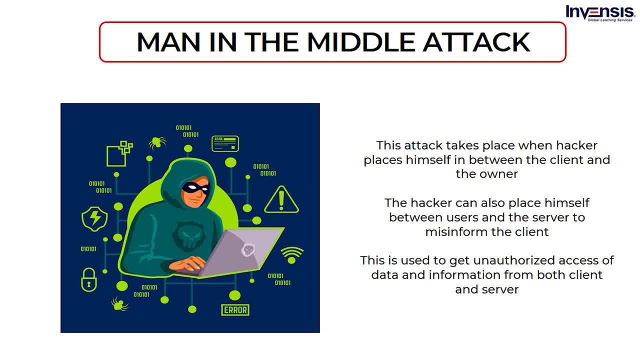 made computer Cortes used to sponge computers class 60ât to telemetry traces. middle cyber attack or MITMA attack occurs when the hacker places himself in between the client and the owner, or between users and the server, or between clients and server to misinform the client. 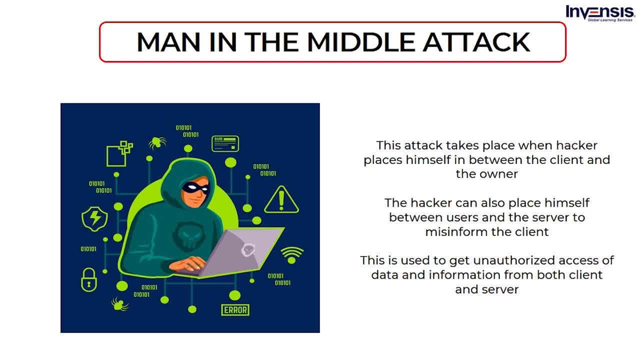 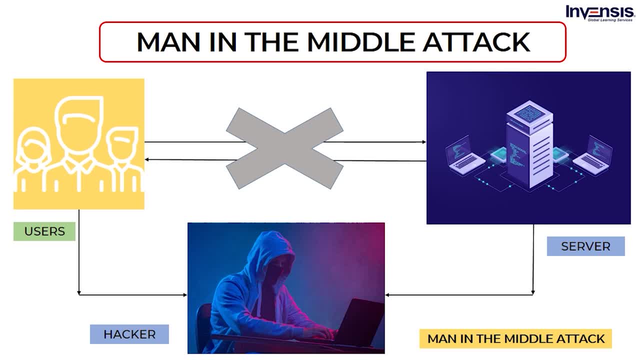 and get unauthorized access to data and information from the system. In this attack, the hacker breaks the communication link between the user and the server. All data and information transfer of both the user and the server goes through the hacker. This gives the hacker unsolicited access to. 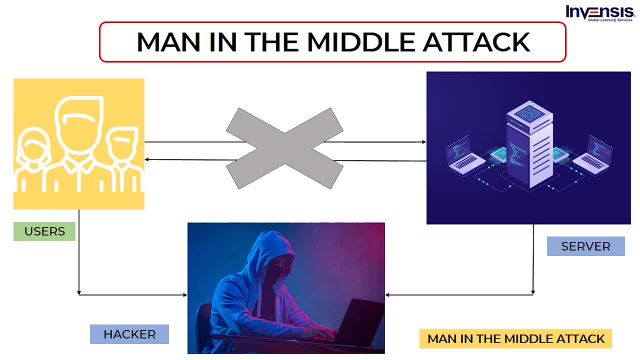 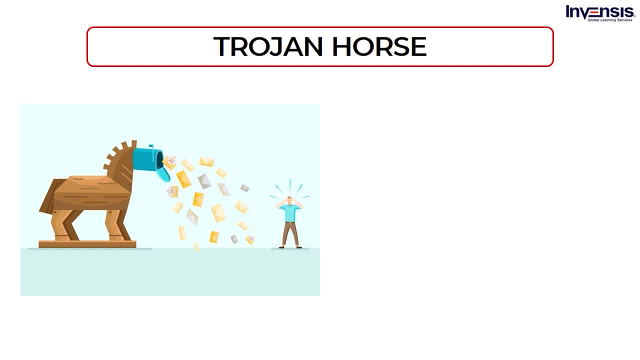 complete information of the whole system. This gives the hacker complete control over the whole system, the data involved and the processes involved in it. We will now discuss the next type of cyber attack, called as the Trojan horse. A Trojan horse, or a Trojan, is a malware program. 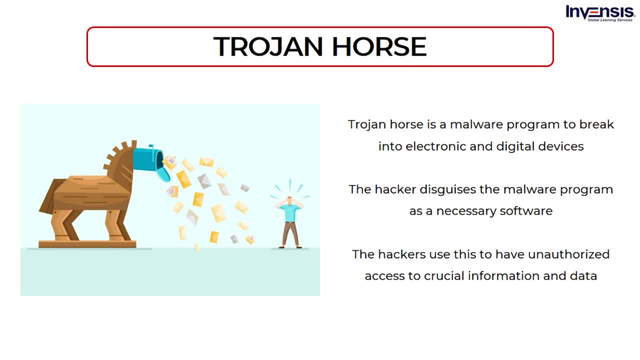 designed by hackers to break into electronic and digital devices by disguising the program with the necessary software. This type of cyber attack is quite dangerous as it helps the hackers to have unauthorized access to crucial information of users, such as their credentials and financial details. 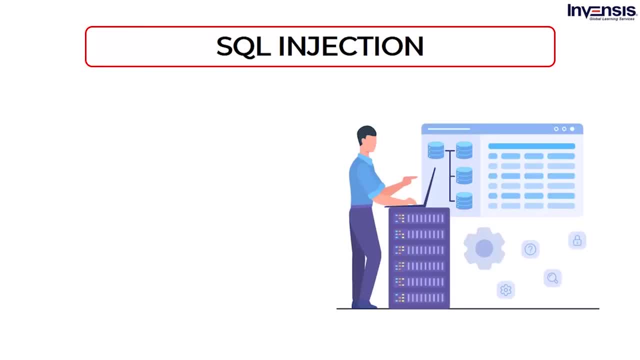 The next type of cyber attack is called the Trojan horse. This type of cyber attack is called the SQL injection. SQL injection is the latest type of cyber attacks being launched by hackers. This includes incorporating malicious data into user's digital device to enable the hacker to 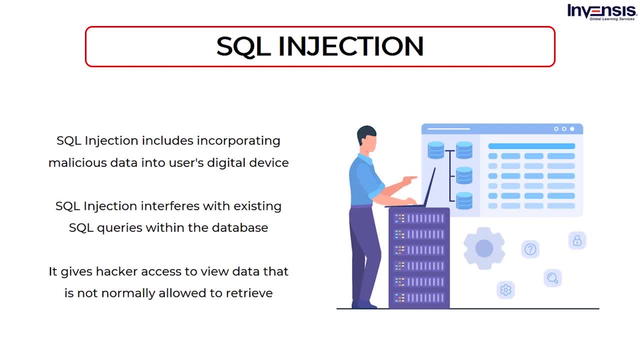 give unauthorized access to all the crucial and confidential information belonging to the user. SQL injection is a cyber attack that allows a hacker to interfere with the SQL queries that an application incorporates into its database. It gives hacker access to view data that is not normally allowed to retrieve. 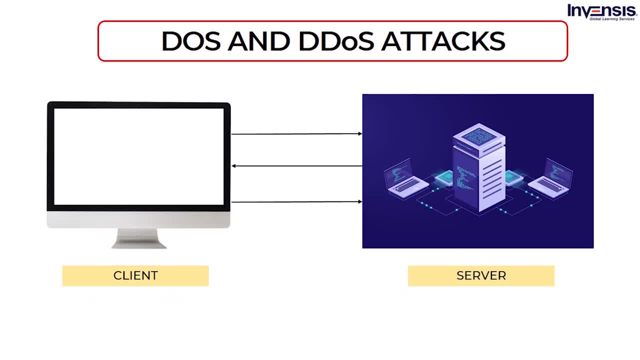 We will now see and understand what DDoS and DDoS cyber attacks are. In a client-server communication system, there are three level handshakes before the data from the server is transferred to the client system. The first handshake is the client's request to the server to load the web page or any. 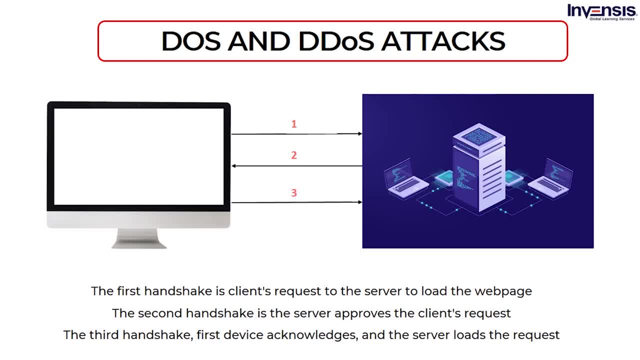 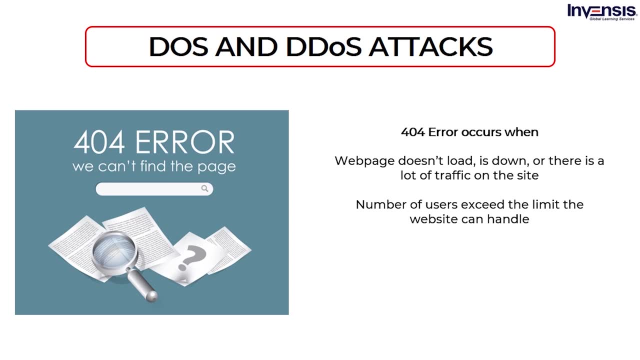 result or any content. The second handshake is where the server approves the client's request, gets ready to load and asks the client device when to load. In the third handshake the first device acknowledges and the server loads the request. Error 404 reflects when a web page doesn't load, the website is down or there is a lot of traffic. 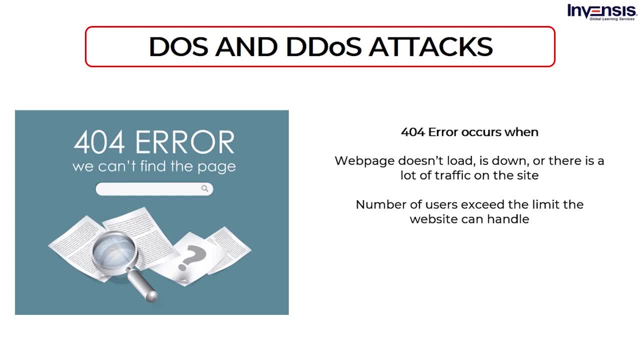 on the website, It is detrimental to the profits of the organization. This happens when the number of users on the website, on that page, exceeds the limit the website can handle. Once it exceeds, the page is down and the users get this error. What happens if someone fakes the number of users? 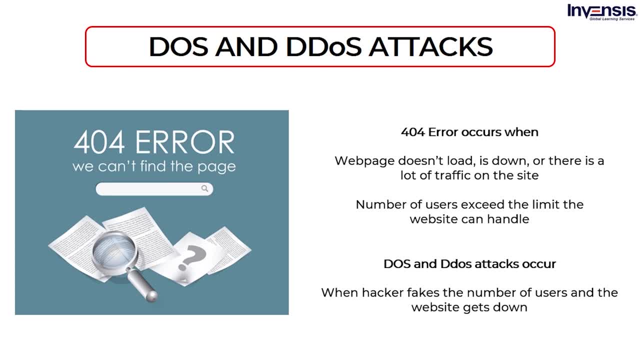 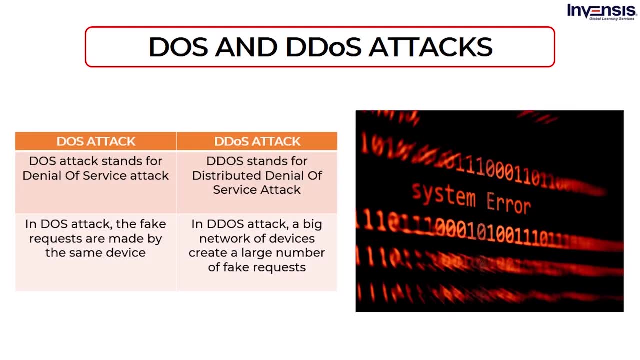 currently using the website and the website gets down intentionally. This is precisely what the DDoS and DDoS attacks are. The DDoS attack stands for Denial of Service Attack. DDoS stands for Distributed Denial of Service Attack. In a DDoS attack, the fake requests are made by the same device to overwhelm the. 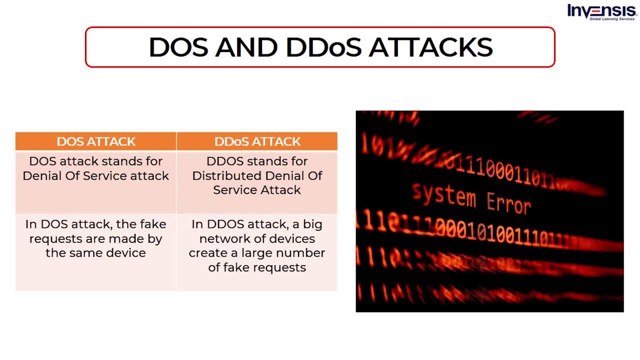 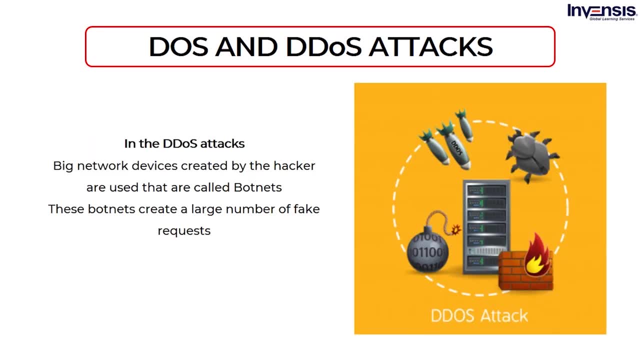 website, causing it to crash. In a DDoS attack, a big network of devices creates a large number of fake requests and together requests the server at the same time. In a DDoS attack, big network devices created by the hacker are called botnets. The botnets create a large number. 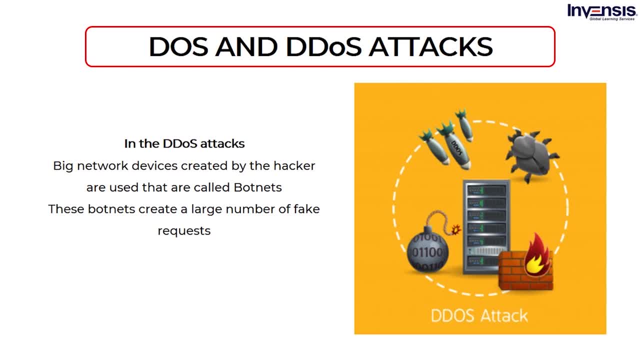 of requests and together all request the server At the same time. one botnet creates one or two requests. In both the attacks, the hacker fakes the number of users currently on the website. Once this number exceeds the limit, the website cannot. 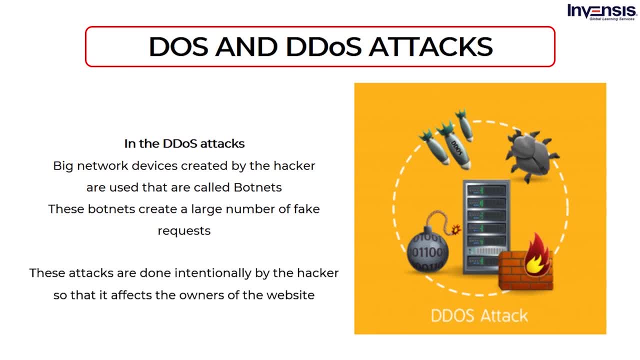 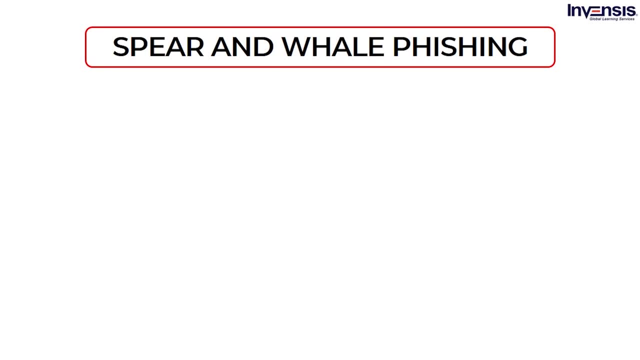 handle this anymore and it crashes down. This crashing is done intentionally by the hacker so that it affects the owners of the website. We will now see spear phishing and whale phishing. In a spear phishing attack, a hacker tries to gain unauthorized access to confidential information. 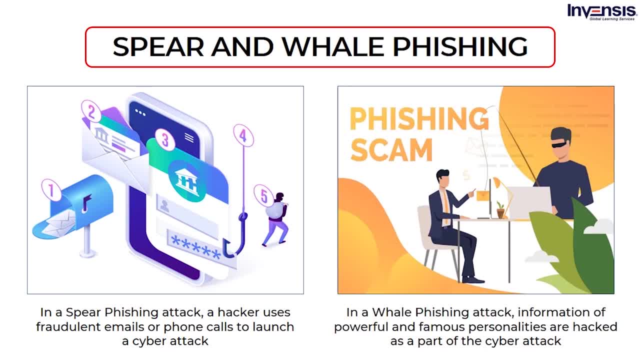 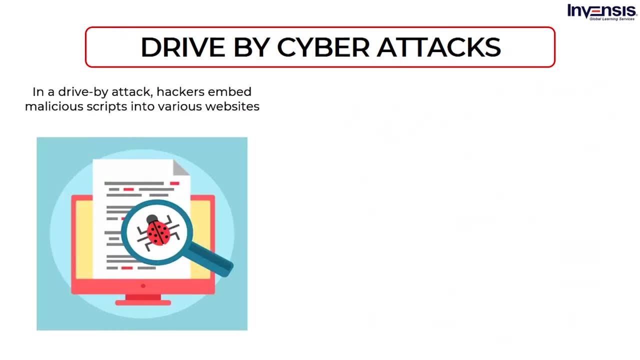 by conducting fraudulent emails or phone calls. In a whale phishing attack, a hacker tries to access confidential and sensitive information of powerful and famous personalities like the chairman and head of organizations. Let us now discuss drive-by cyber attacks. In a drive-by attack, hackers embed malicious 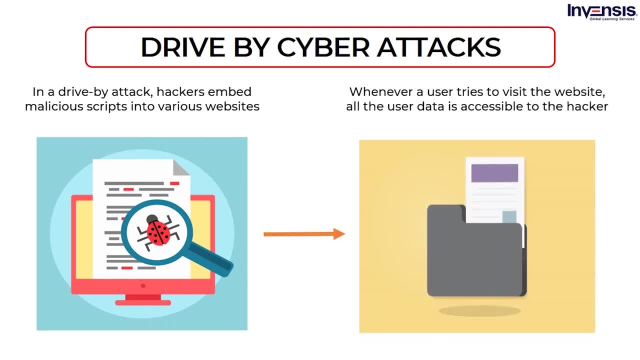 scripts into various websites. Whenever a user tries to visit the website, all the user data is accessible to the hacker. Because of these malicious scripts, the system gets corrupted, giving unauthorized access to data and information to the hacker. The next attack is a spear phishing attack. A hacker tries to access confidential and sensitive. 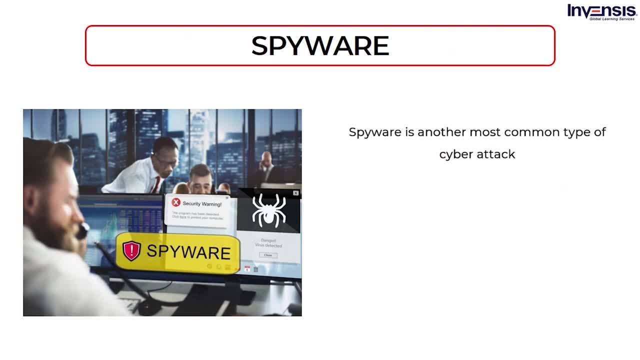 type of cyber attack is called the spyware. Hackers use cyber attacks called spyware, which is unwanted software, to infiltrate into a victim's computer in order to have access to their sensitive information and internet usage data. It is a type of malware that uses malicious 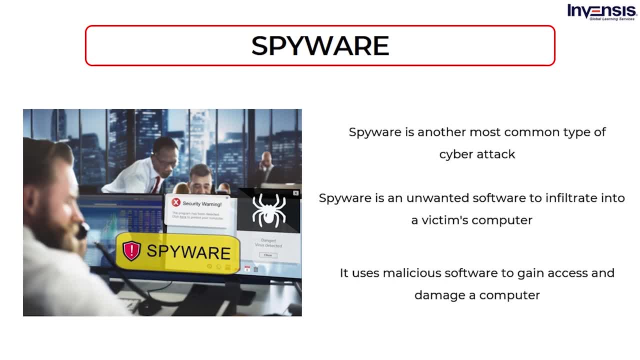 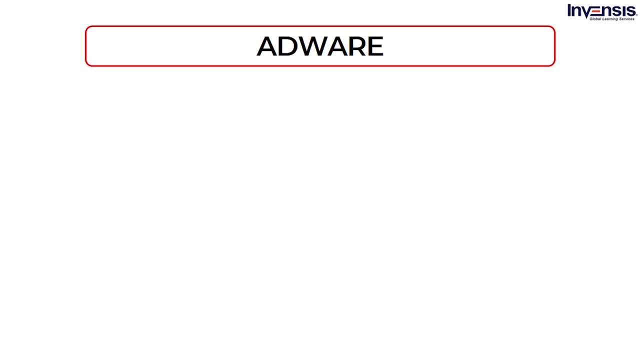 software to gain access and damage a computer without the knowledge of the user. There are again four types or categories of spyware, commonly called as: 1. Adware, 2. Keyboard loggers, 3. Trojans, 4. Mobile spyware. The next type of cyber attack is called the adware, The cyber. 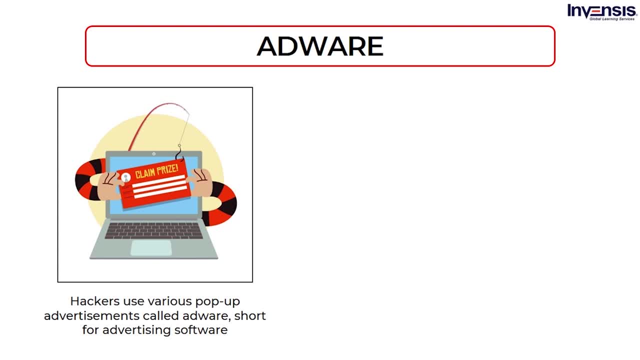 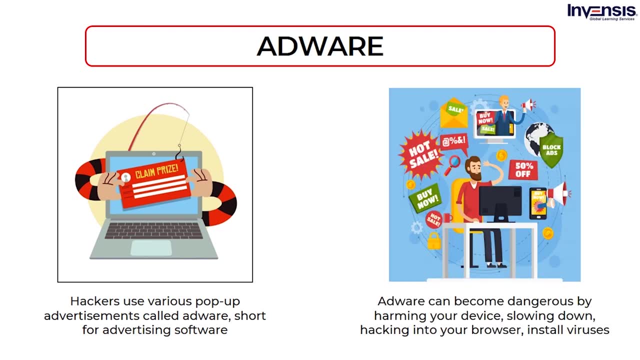 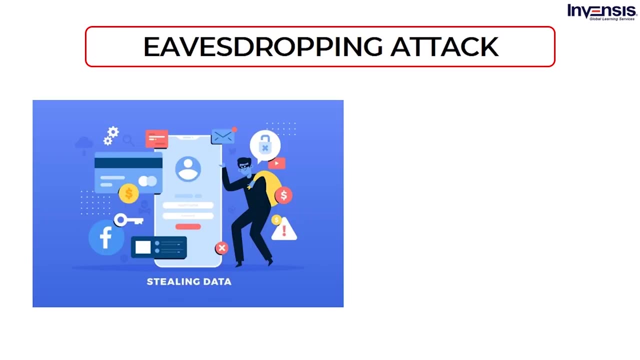 attacks where hackers use various pop-up advertisements to show up on a computer or mobile device are called adware, short for advertising software. The adware can become dangerous by harming your device, hacking into your browser, slowing down the device and install viruses or spyware or both. The next type of cyber attack is called the. 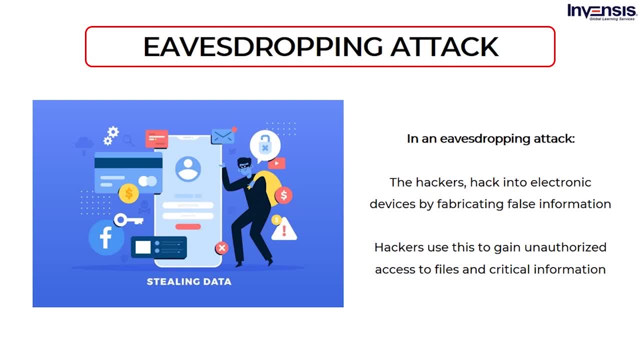 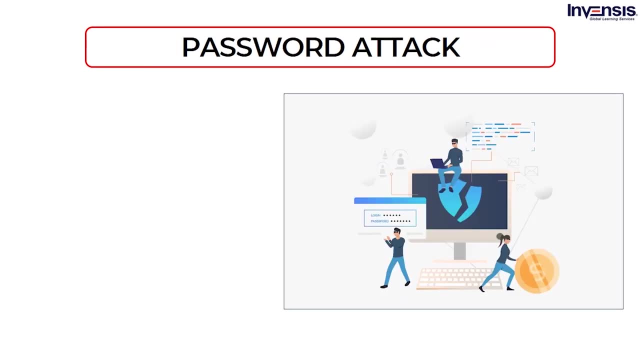 eavesdropping attacks. When hackers launch a cyber attack by hacking into cell phones, computers and laptops by fabricating information in those devices, it is called an eavesdropping attack. This attack is conducted to gain unauthorized access to files by cybercriminals. The next type of cyber attack is called the. 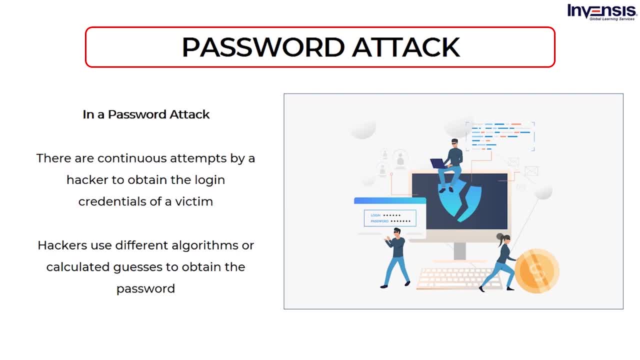 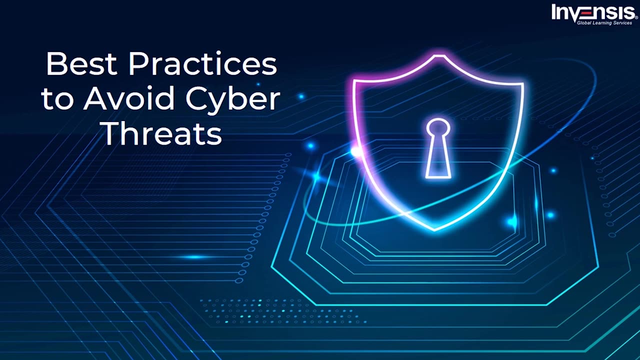 password attacks. A password attack involves continuous attempts by a hacker to obtain the login credentials of a victim or user. Many hackers use different algorithms or simply make calculated guesses to obtain the password in the shortest time possible. 4. Password. We will now discuss the most crucial part of today's discussion. 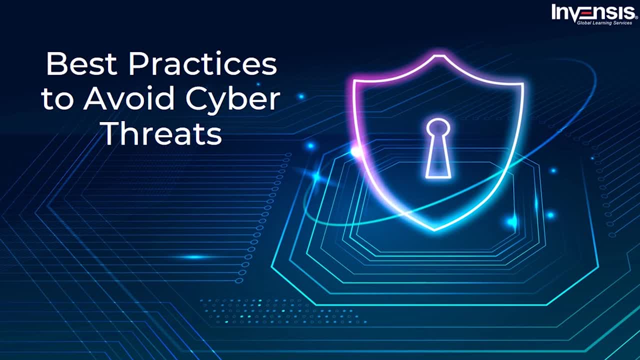 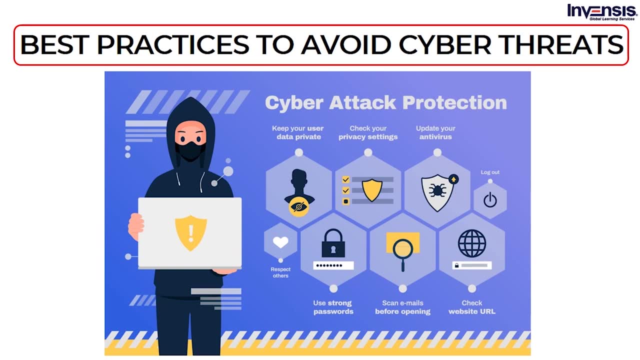 Basic Practices and Methods to Avoid Cyber Attacks. Best practices and methods to avoid cyber attacks include the steps and methodologies involved to keep oneself and any organization on the whole safe and secure, both internally and from any external threats, be it cyber attacks or any viruses or computer worms. 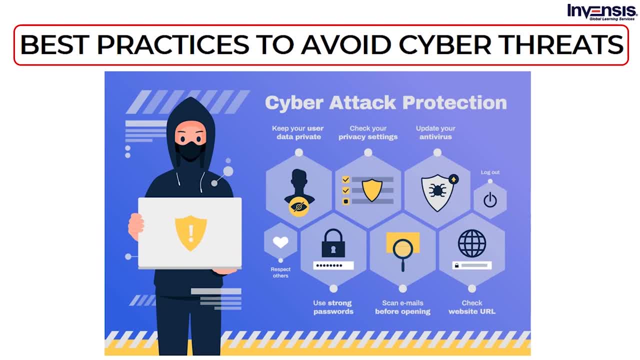 etc. These practices and methods help in a smooth and safe operating environment and include: 1. Keep your user data private. 2. Check your privacy settings. 3. Update your antivirus. 4. Use strong passwords. 5. Scan emails before opening. 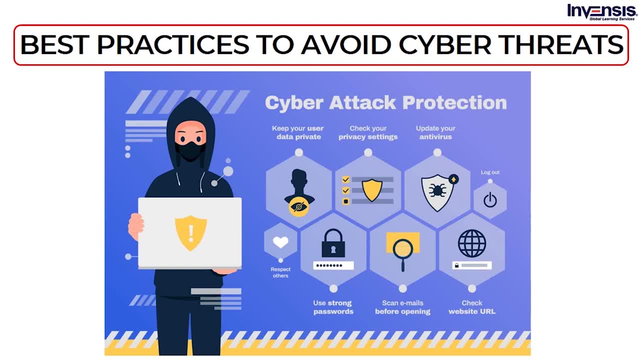 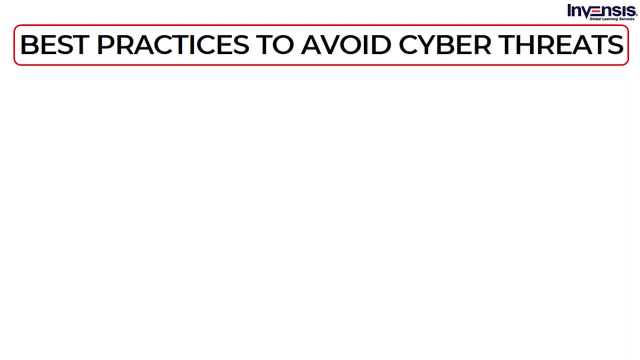 6. Check website URL. 7. Log out as in when required. 8. Respect others. Let us now look into each of these in detail. Data Privacy: Having user data privacy is the first step against cyber threats. Always make sure that you keep your data private. 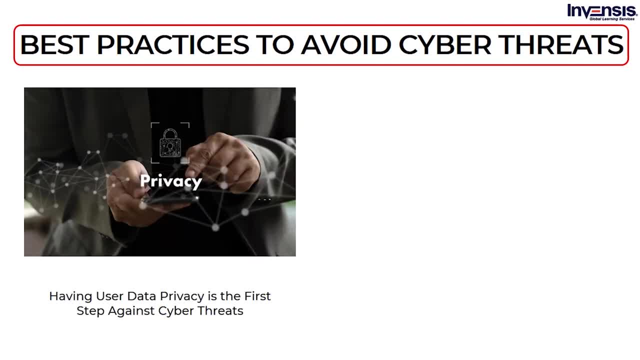 Always make sure that you keep your data private. Always make sure that you keep your data private. Always keep your data private. Always make sure that you keep your data private. Keep your data private. Always keep your data private. Keep your data private. 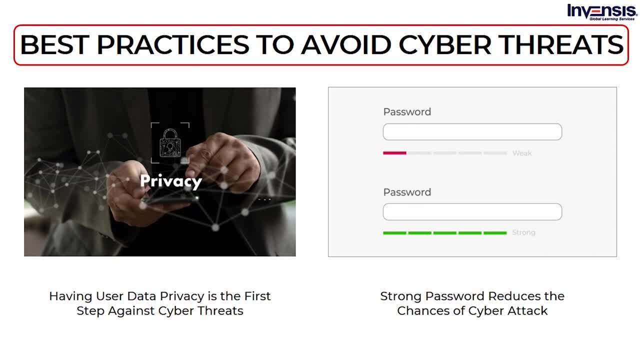 Keep your data safe on all platforms. Keep your data safe on all platforms. Keep your data safe on all platforms. Any user by default should not spread the word unauthorized. Any user by default should not spread the word unauthorized: проис اس moi. 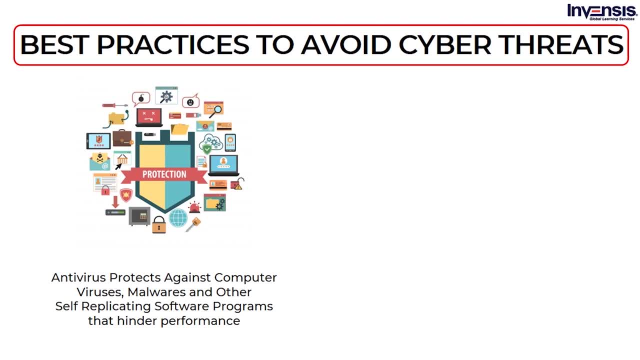 rolled personal. No viruses and computer worms and other programs developed in order to deliver a cyber attack. Scan emails. Scanning emails before opening them prevents any dangerous email-embedded cyber threats from harming the userIt is highly recommended to scan your emails before opening. 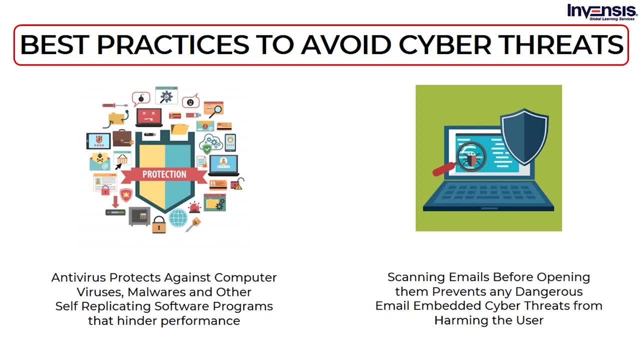 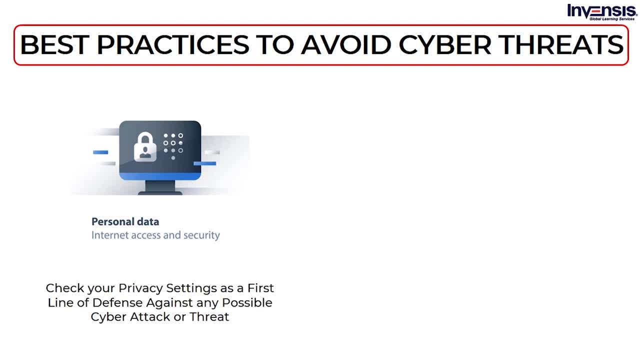 them. This helps, in a way, to avoid the chances of various email hacking attacks usually used by hackers. Privacy settings: Check your privacy settings as a first line of defense against any possible cyber attack or threat, Maintaining strong privacy settings for all your work. 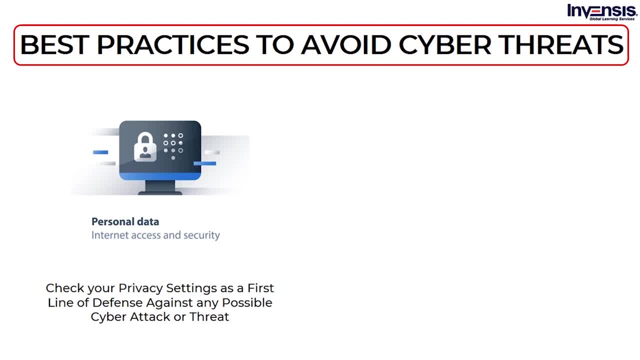 be it on mobile devices or laptops or computers, act as the first line of defense against hackers. Website URL Cross-checking the website URL is very important to avoid opening any malicious website. A website that starts with HTTPS is far more secure than the ones that. 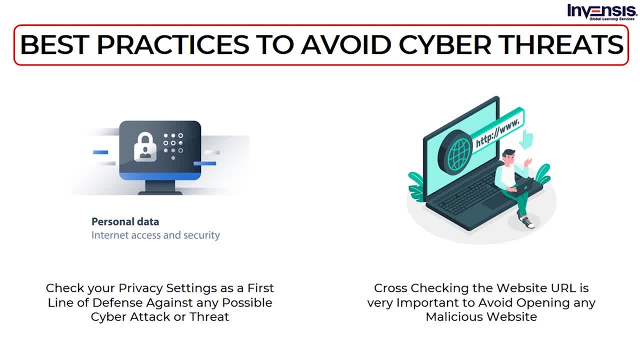 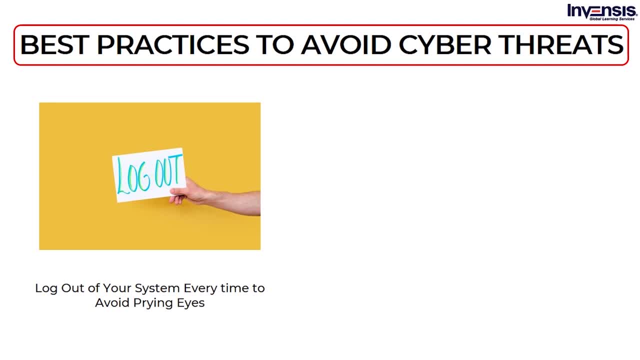 start with HTTP. The additional protection provided always counts in the advent of any cyber attack. Log out. Log out of your system every time to avoid prying eyes. Every time you complete your work and don't intend to use the system, log out of the system. This is a preemptive measure.